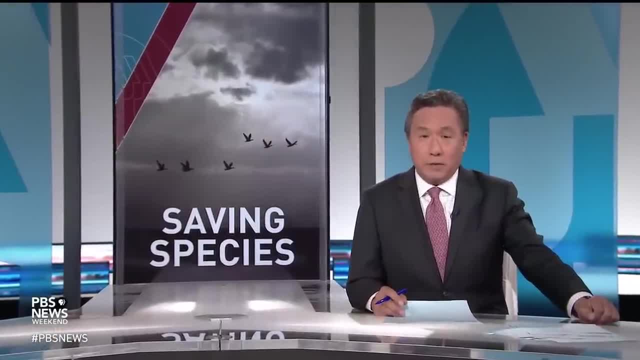 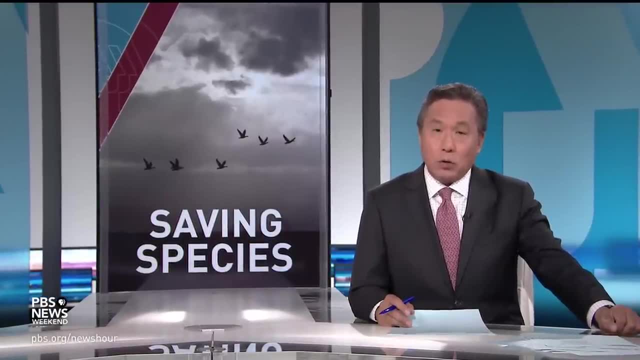 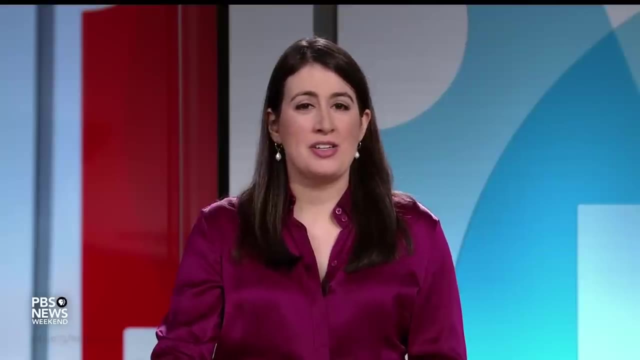 As the climate crisis worsens, so does pressure on wildlife. New research indicates that the population of nearly half of all animal species is declining And, as Ali Rogin reports, among the most affected are birds. ALI ROGIN, If you're accustomed to waking up to the sound of them chirping or watching, 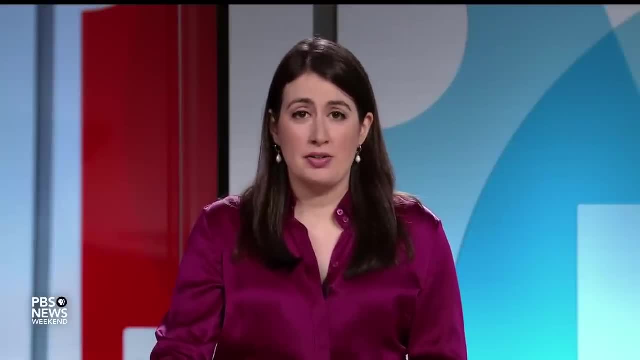 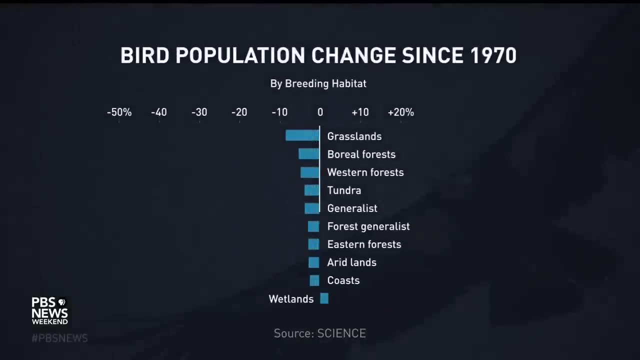 them flock to the feeder outside. you might not realize it, but birds are in trouble. The number of birds in North America has declined by three billion in the last 50 years. That decline has hit some species of the animal harder than others, with birds living in Canadian 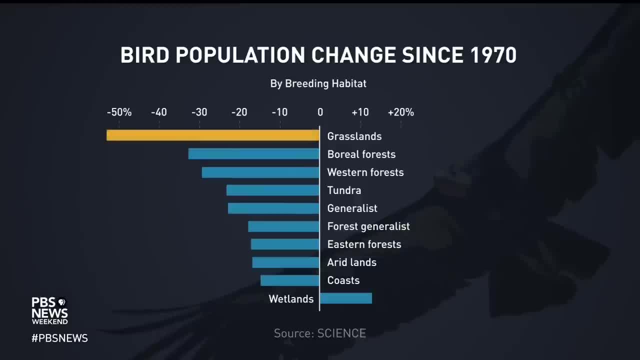 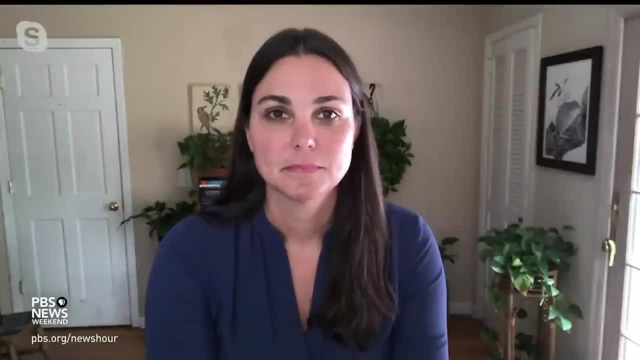 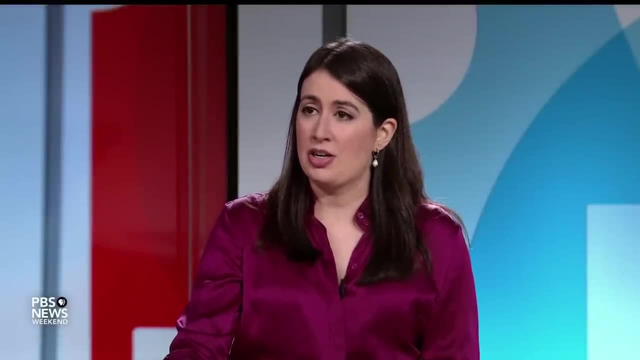 and American grassland habitats experiencing the biggest drops in population. Joining me now is Brooke Bateman, director of climate science at the National Audubon Society. Brooke, thank you so much for joining us. Two-thirds of North American bird species are teetering on the edge of extinction. Why? 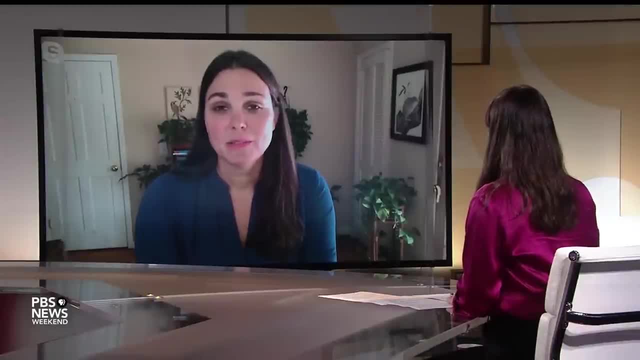 is this? What environmental factors led to this BROOKE BATEMAN National Audubon Society? Yes, so we have lost 30 percent of our birds since 1970. And a lot of the changes have been caused by climate change. And a lot of the changes that we have seen across North America are due to human changes in the landscape, such as loss of forests, conversion of grasslands to agriculture, So we have seen a lot of habitat loss that has really affected the birds in North America. 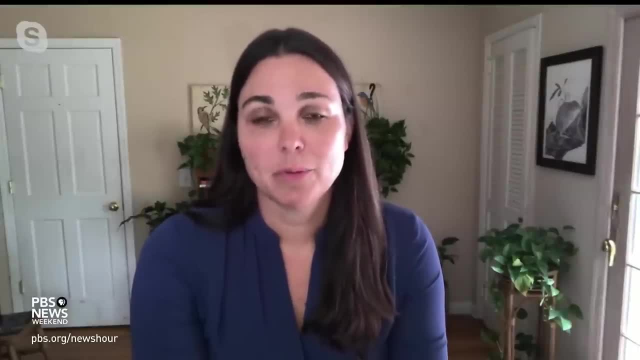 where they have less habitat than they used to back in 1970 and prior to that, ALI ROGIN. And how much of this is attributable to climate change? BROOKE BATEMAN National Audubon Society. So we are already seeing effects of climate. 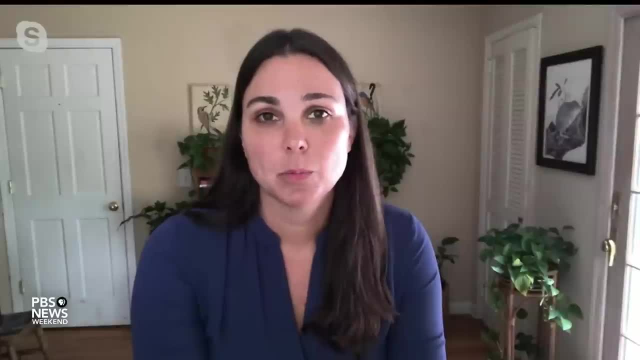 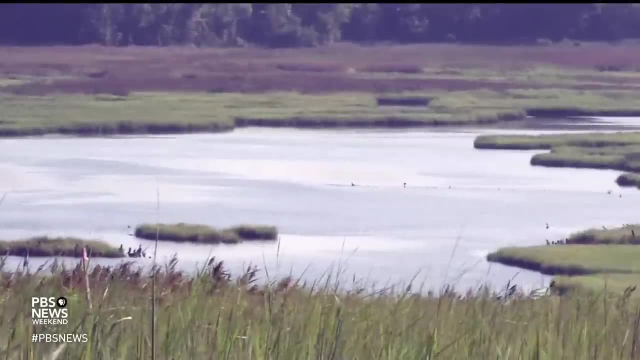 change, And what we're actually seeing is sort of these two effects working together against species. So the loss of habitat combined with climate change is making it trickier for birds to find places that have ideal conditions for them to survive. So we're already seeing 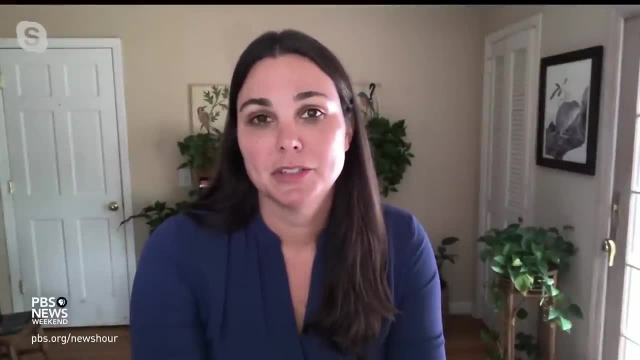 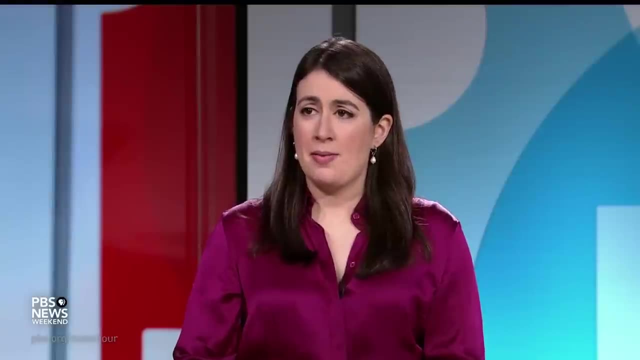 birds move because of climate change and trying to find new locations to move into, And that's tricky when there's not a lot of habitat because things have been altered on the landscape from what they have been used to. ALI ROGIN National Audubon Society And tell us a little bit about the role that? 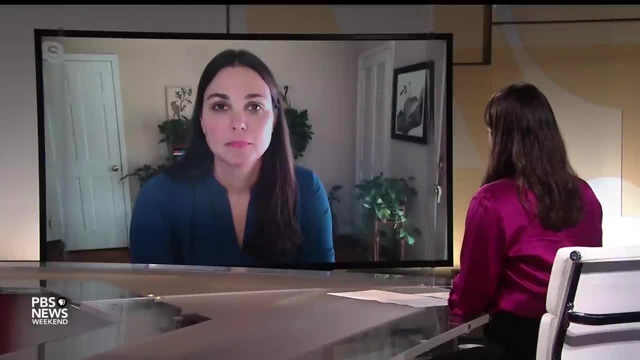 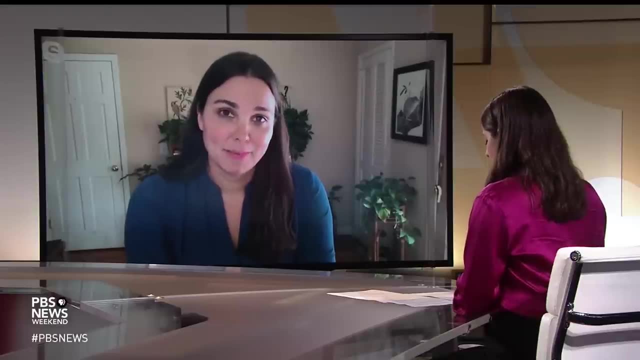 birds play in the ecosystem and what might happen? What are the detrimental effects if their populations continue to decline? BROOKE BATEMAN National Audubon Society. Yes, birds are really integral for the ecosystem. At Audubon we say: birds tell us. because birds tell us what's happening in the ecosystem. 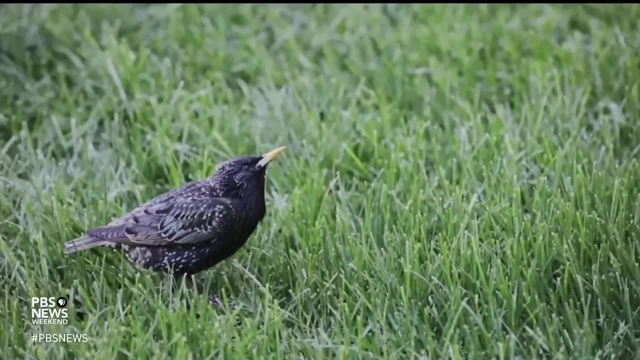 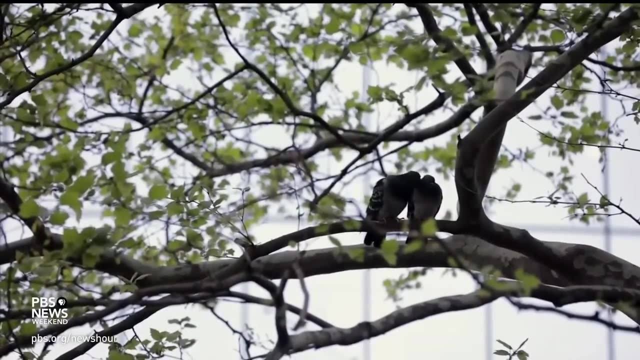 And they really are tied to the changes that we're seeing, And so birds are really important for things like insect control. They really help our crops, including our coffee crops that have insects that come help, And by eating the insects they help those crops survive. They also keep away some of our invasive species, the insects, like emerald ash borers. They're really important for pollination. So some of the key things that we need from pollination brings us our vegetables and our fruits And birds are key for that, along with insects. 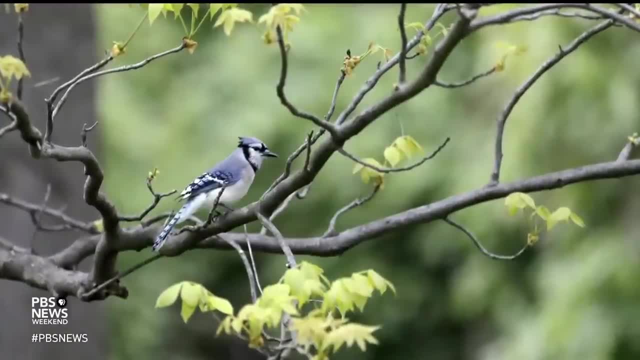 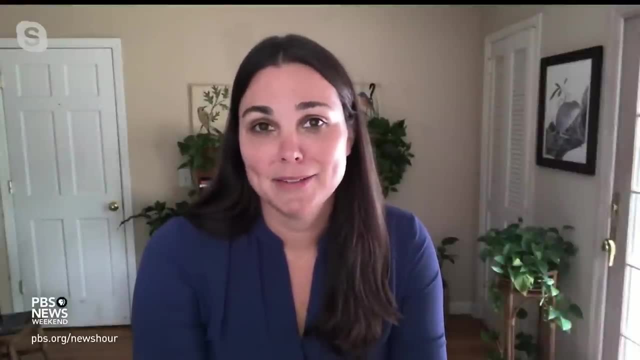 And they also do other things. So blue jays, for example, are one of our what we call ecosystem engineers, because when they pull acorns off the ground from oak trees they can actually move those hundreds of miles and build forests. So they're important for the movement and 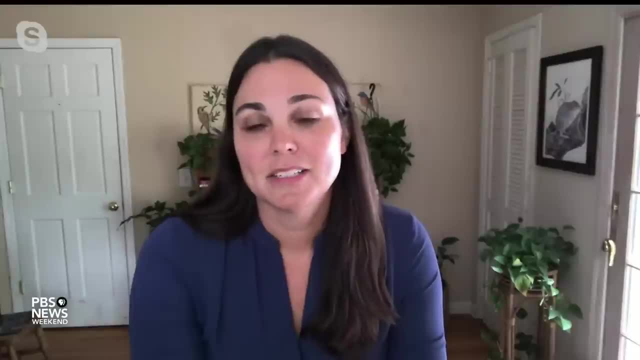 the growth of new forests. So birds just do a ton for us, And if we didn't have them we would lose a lot of those ecosystem services. ALI ROGIN National Audubon Society, Talk to us about the efforts on the federal 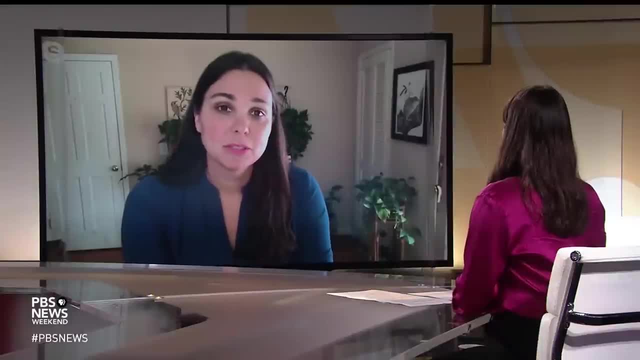 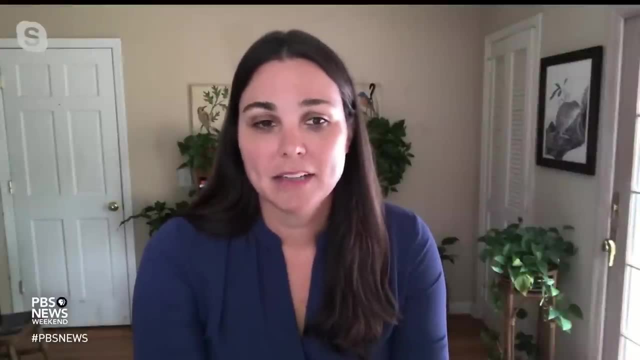 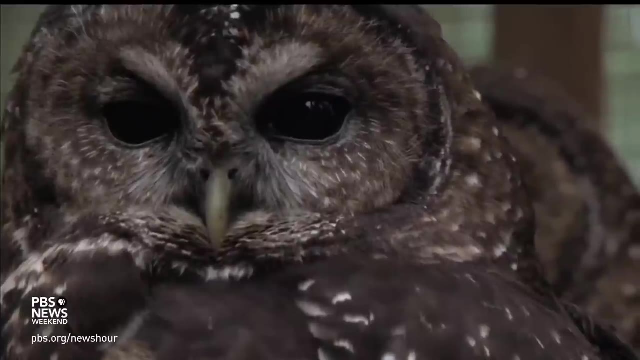 level to conserve these species. GABRIELA CARVALHO. Yeah, So the Migratory Bird Treaty Act is an act that helps protect migratory birds and protects them, And so that's been a really important act that has helped birds and keep them protected within North America, as well as the Endangered Species. 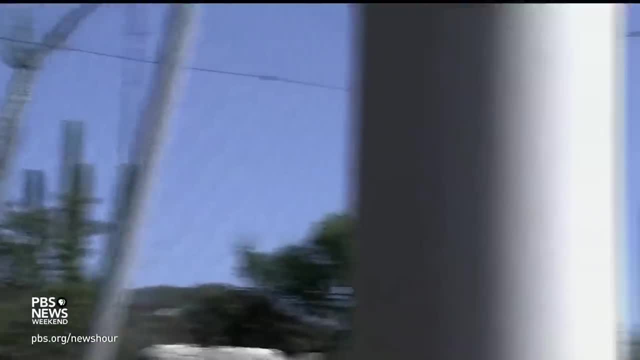 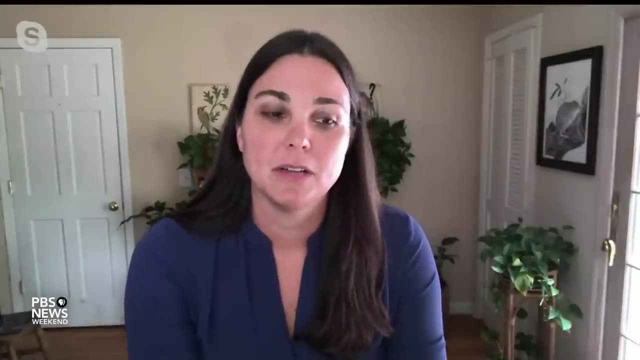 Act for some of our species that are endangered, to really make sure that they have the safety that they need out in the places that they live. So those are two really important federal policies that help protect birds, AMNA, NAWAZ- And I know a lot of the efforts right now. 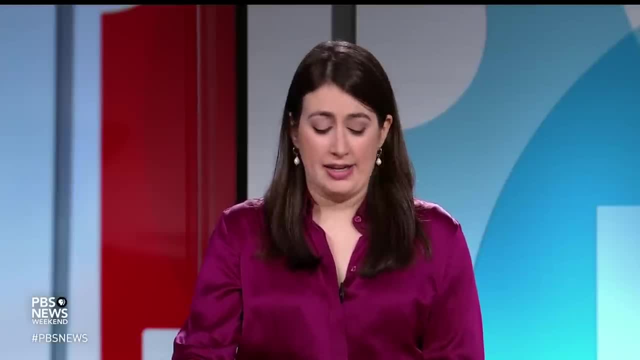 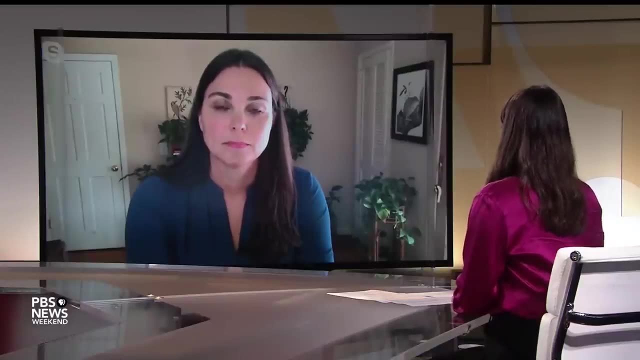 hour about keeping birds off that Endangered Species Act list, But what additional steps would you like to see in terms of preserving and renewing these species populations? Yeah, so I think one of the biggest things that we can do is try to help bring back certain 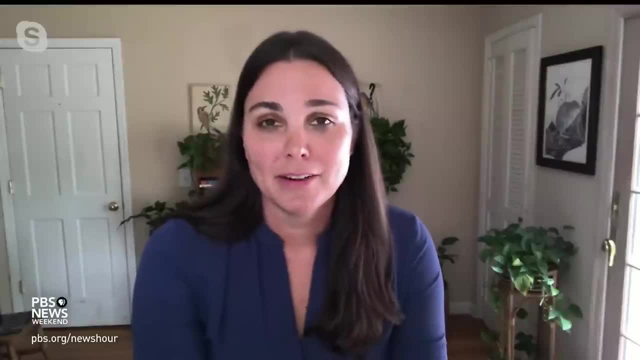 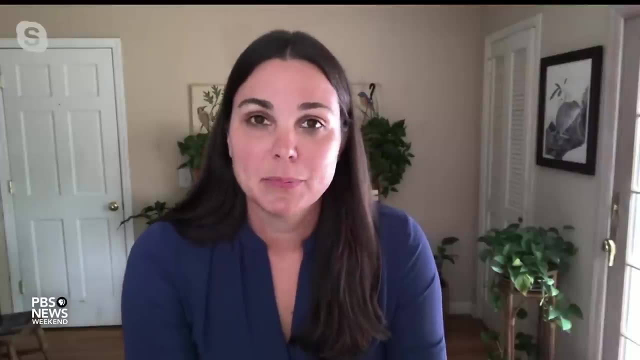 habitats And restoration efforts are really going to be key here, But there are things that you can do even in your own backyard, So one of the things that I think is the most exciting and promising is planting native plants and reducing the amount of grass that you have in your backyard. 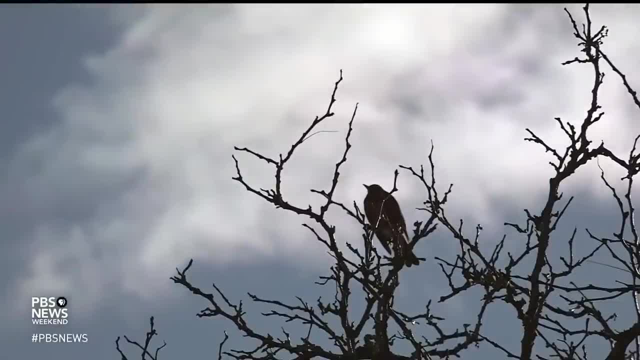 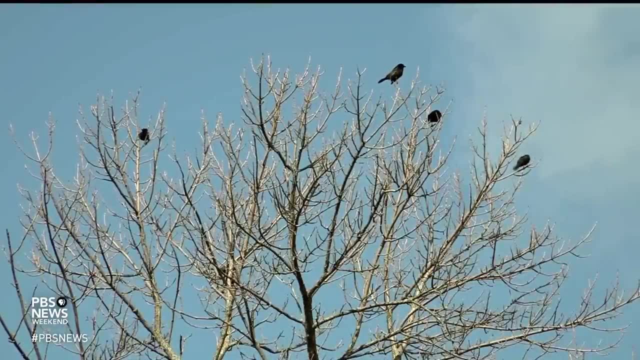 and putting more native plant species, because that will provide habitat for birds and food for birds, And also it actually has a wonderful side effect that plants actually store carbon in their matter And so that helps pull carbon out of the atmosphere- carbon dioxide- So it also helps with. 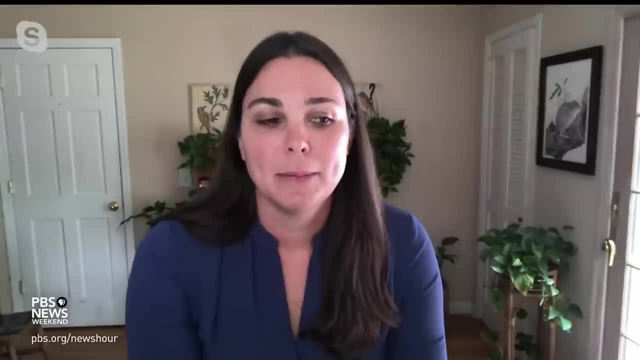 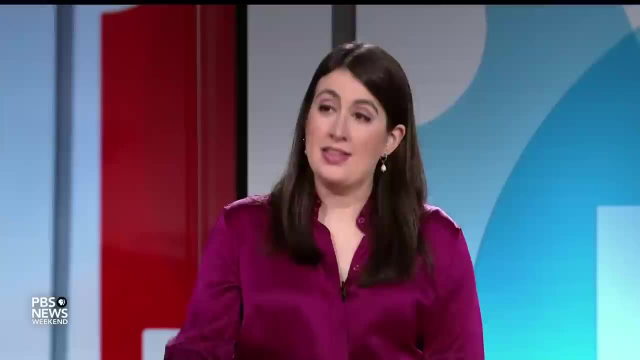 climate change. So it's kind of a win-win to rely on these ecosystem native plants and habitats. that will benefit birds and help stabilize the climate, And the Audubon Society has been doing a lot to get it going. Individuals involved as well. I mean the Audubon Society has been. 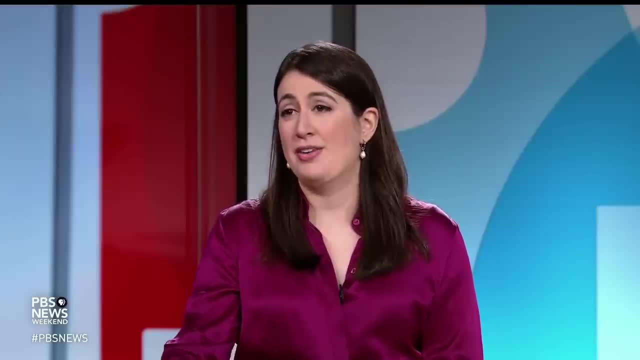 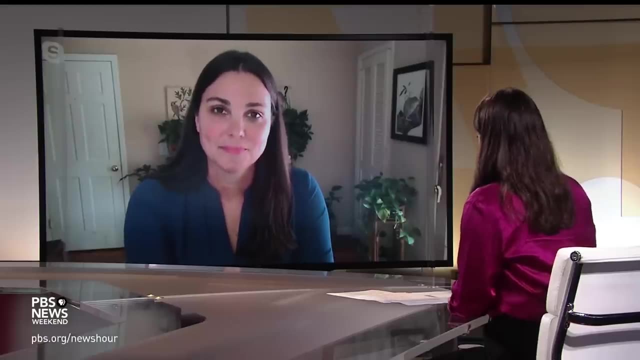 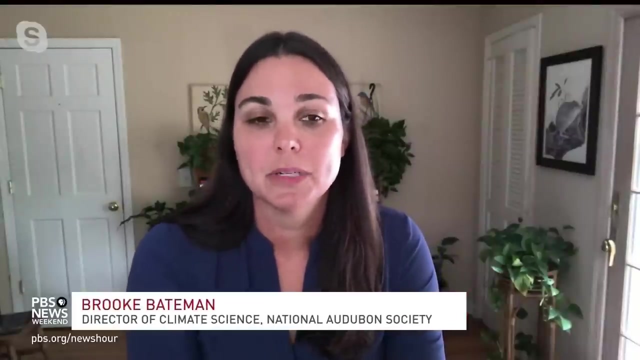 studying birds since it was founded about a century ago. But now you have a lot of kind of open source resources for folks, including the Climate Watch program. Tell us about that and how it's helping advance our understanding of birds. Yeah, So at Audubon we study how climate change affects birds. We put out a report in 2019 that. showed that two-thirds of birds in North America are at risk of extinction because of climate change, And so we really wanted to track how that was going to affect birds, And so we did a lot of research on that. And we did a lot of research on how that was going to affect birds, And so we did. 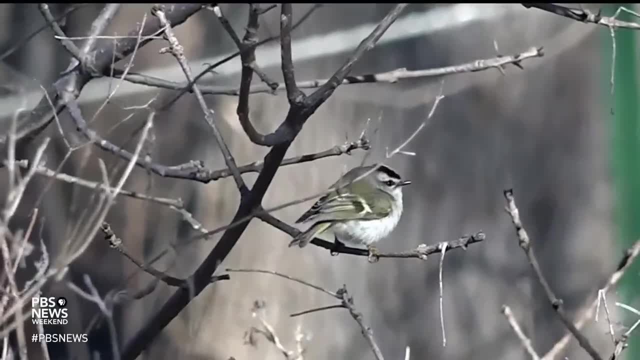 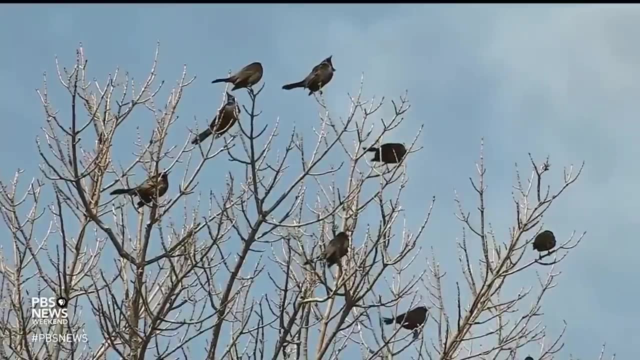 a lot of research on how that was going to affect birds And so we did a lot of research on how that on the ground in real time, And Climate Watch is having volunteers across the country go out and count birds and look for birds- And what we're doing as scientists: we're studying and looking. 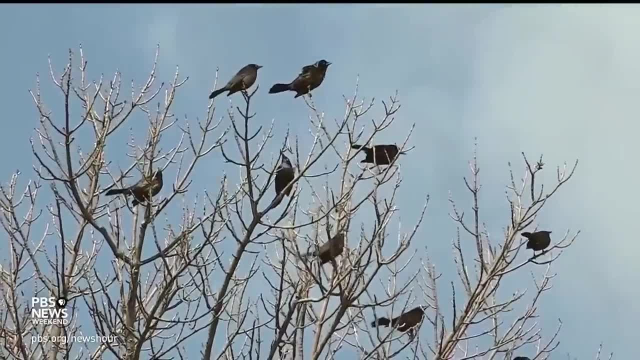 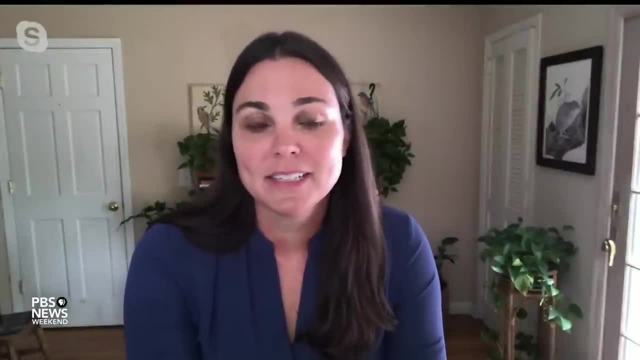 at how these birds are actually shifting where they live because of climate change, And so we're looking at climate change as it's happening. Climate change is not a far-off problem that's happening only with polar bears. We're actually finding that the birds are changing where they. 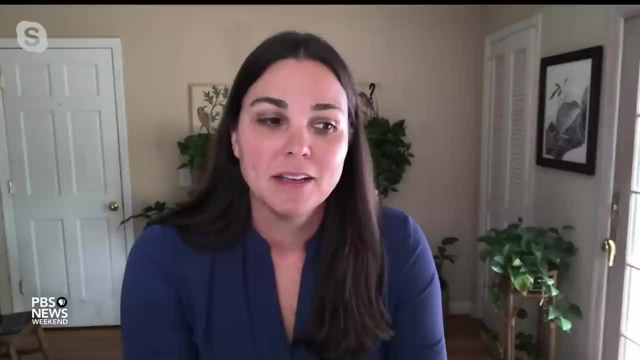 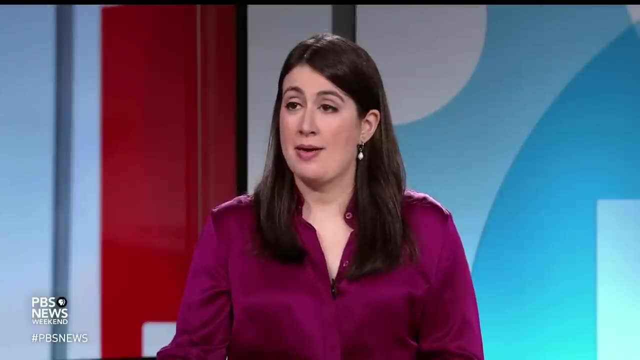 occur because of climate change, And that's because of the Climate Watch program. It's one of the ways that we're able to understand that climate change is already affecting the birds that we love in our backyards- AMNA, NAWAZ- And of course, we're talking about all of 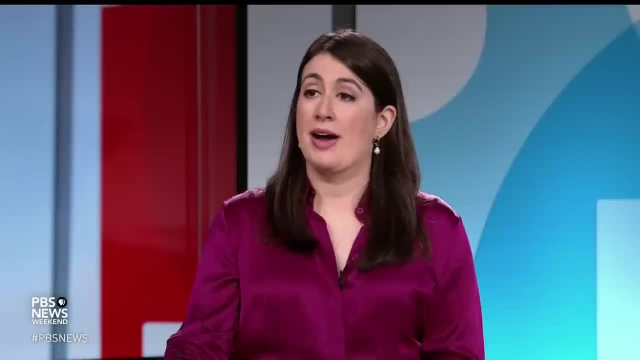 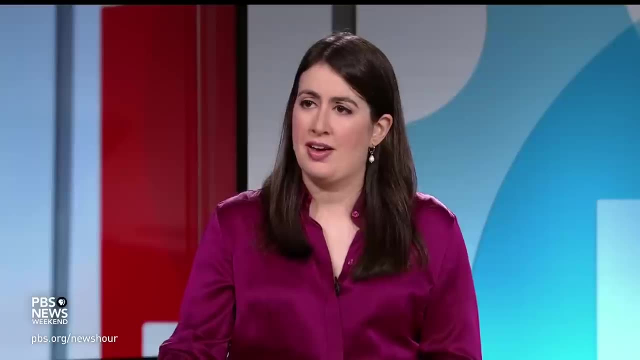 these species that are endangered. But there are some bright spots, it seems, in some of these recent reports, including waterfowl populations have actually been on the rise And that seems to be, kind of ironically, thanks to the efforts of hunters and fishermen. 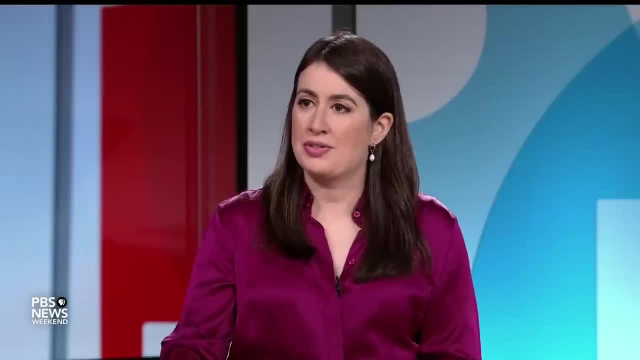 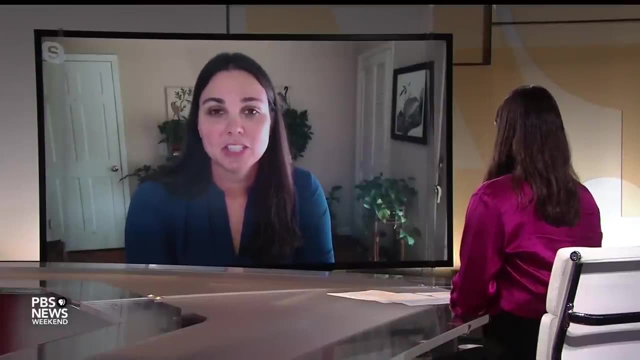 I'm wondering if you can talk about that and any other notable grassroots efforts to preserve certain species. AMNA NAWAZ. Yeah, I think waterbirds are a wonderful example of how, when we take conservation actions into our own hands and put some funding into. 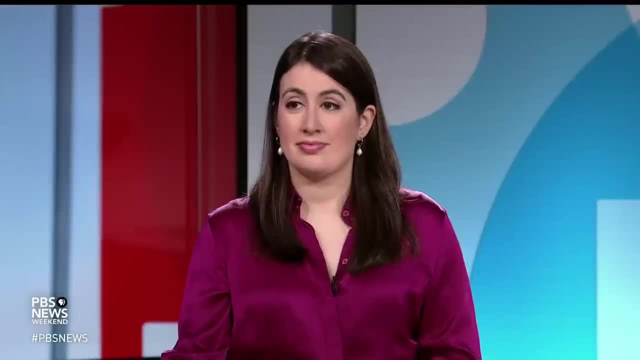 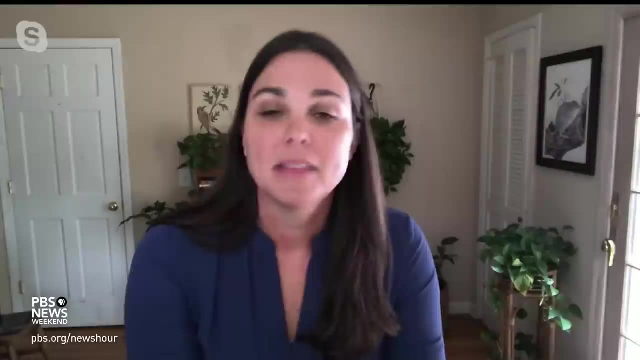 it we can really make a big difference And the funding that's been coming in through hunters, as well as duck stamps, which hunters need to acquire before they hunt- but anybody can buy a duck stamp- that money goes back into the system. 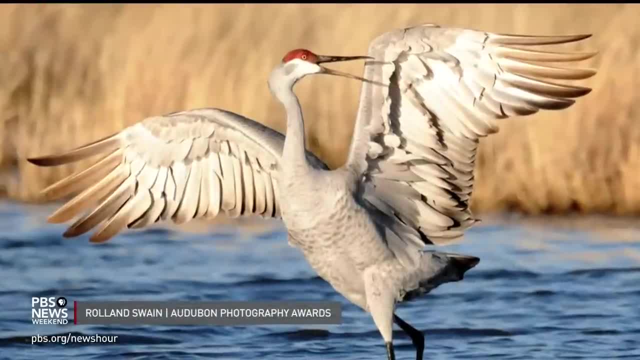 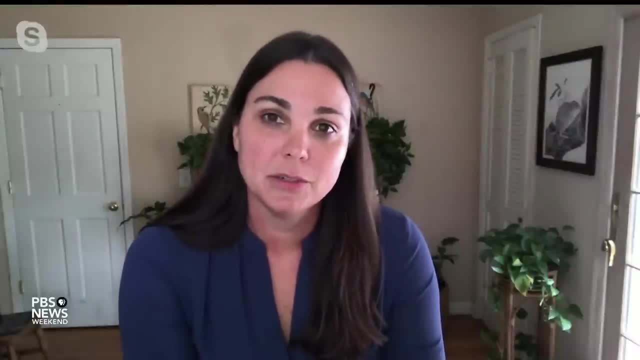 And the Fish and Wildlife Service helps establish habitats and do conservation efforts that have helped waterbirds do so well. So I think it's a great model to show that if we know what we need to do, we can do it, And if we know what we need to do, we can make a big difference.